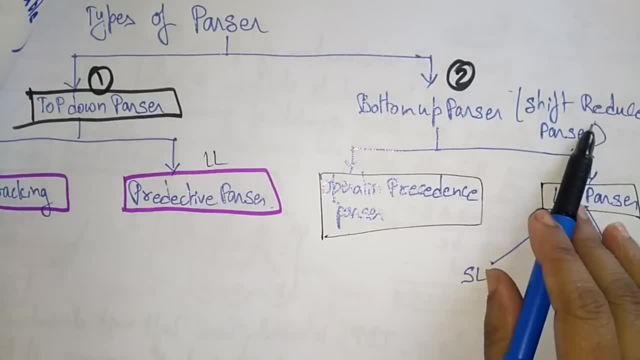 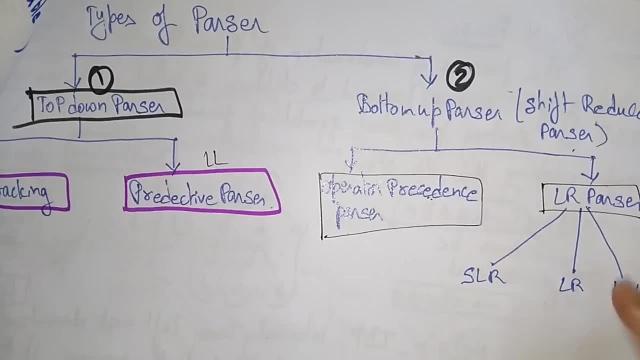 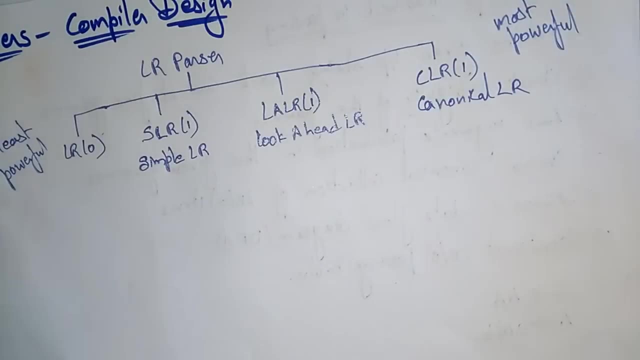 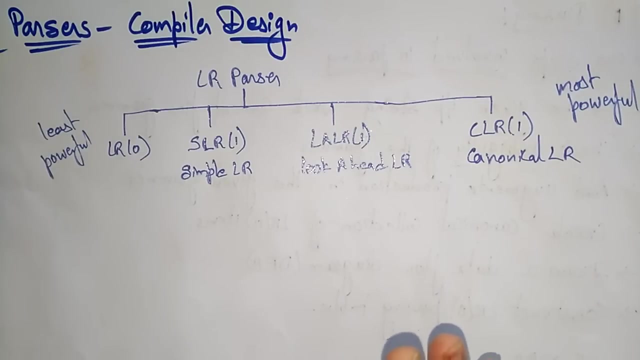 LL parser, that is a predictive parser, shift, reduced parser, operator parser. So these comes under the bottom up and these two are the top down parser. Now let's see the another type of bottom up parser. This is LR parser. Okay, so now let's see what is this LR parser? LR parser is again of. there are different types are available. Okay, so mainly three widely used algorithms available for the LR parser. for 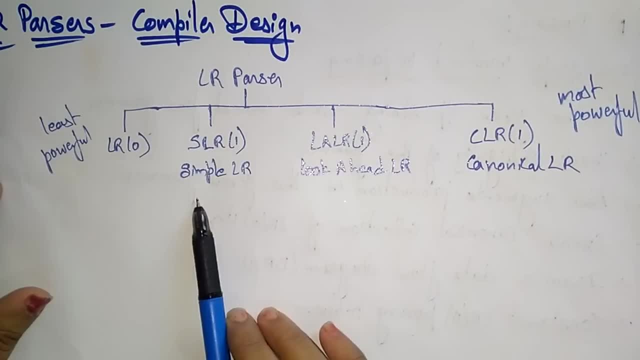 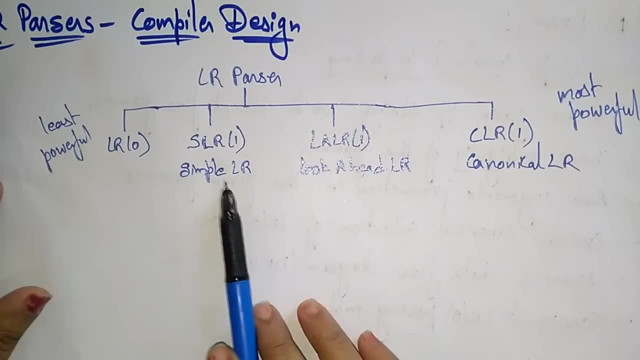 constructing. So those are SLR, LALR, CLR. Okay, LR parser is divided into LR0, SLR, LALR, CLR. Okay, SLR means simple LR, LALR is- look ahead- LR and CLR is a canonical LR. So, from going this side, LR0 is having the least powerful and whereas CLR 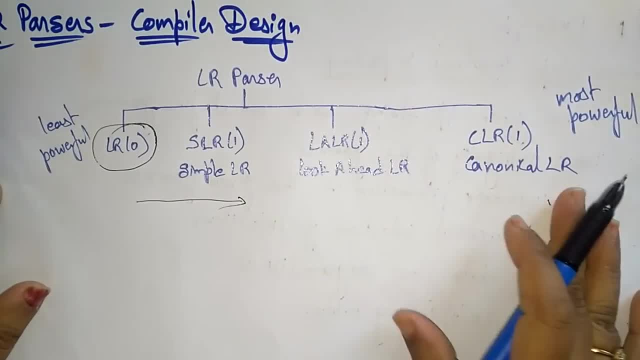 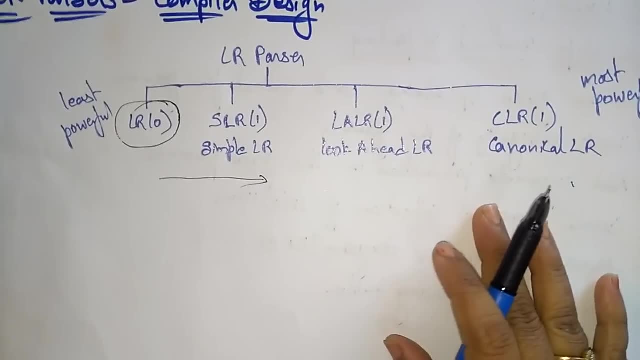 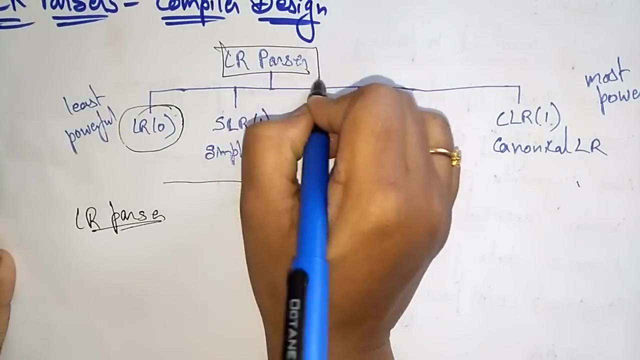 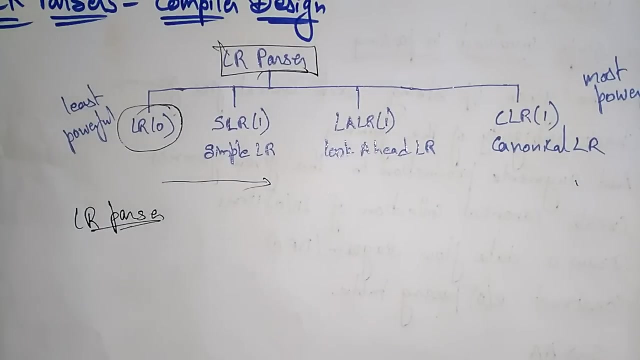 is the most powerful. Okay, so, when compared to this, from left to right, the LR0 is having the least powerful and CLR is most powerful. So what is this LR parser? So in this video, I want to explain what exactly the LR parser was. Okay, so, LR parser. and in the next, in the coming videos, we'll see, with an examples. So LR parser. LR parser is a non recursive shift. 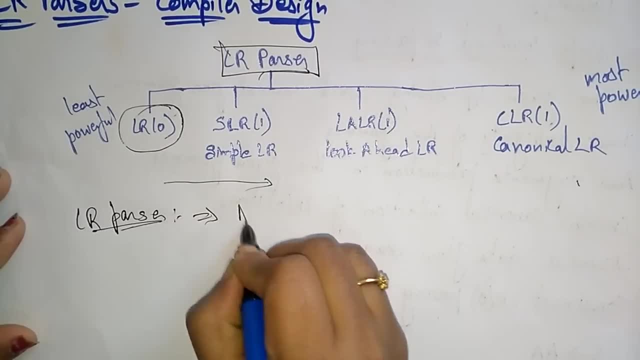 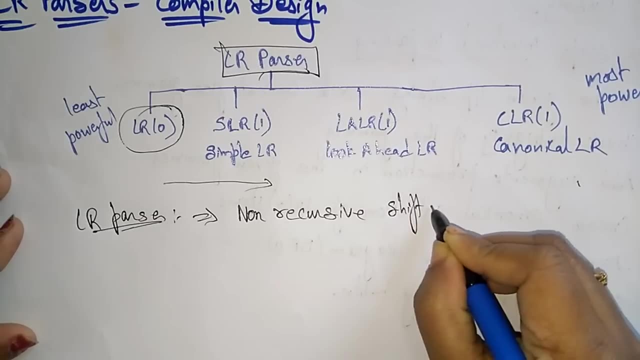 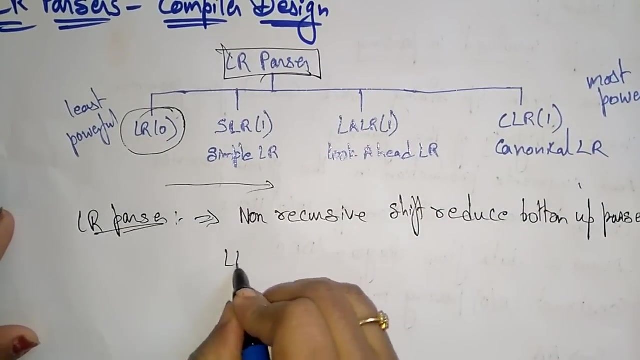 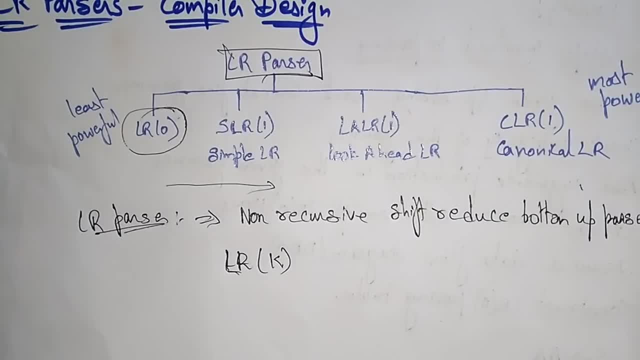 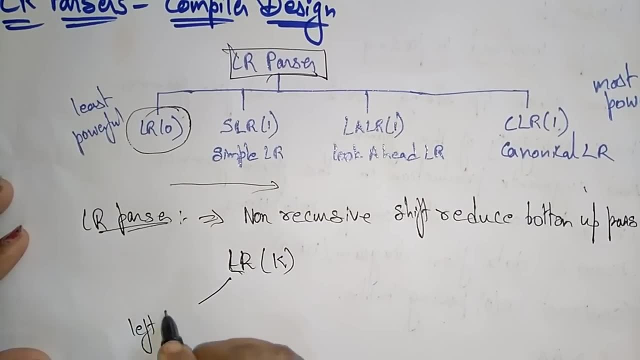 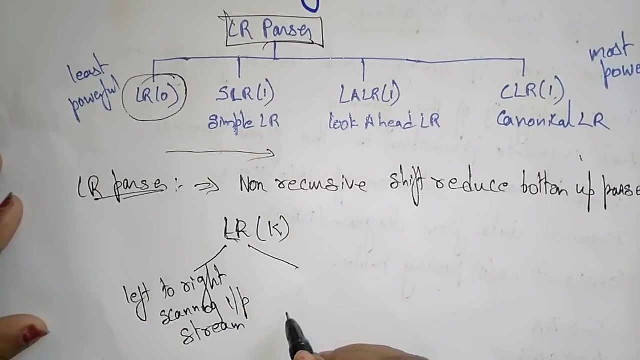 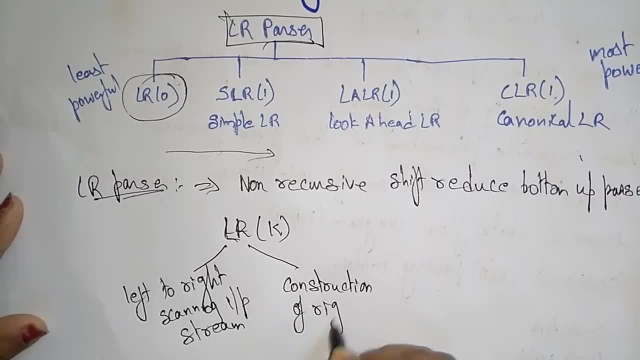 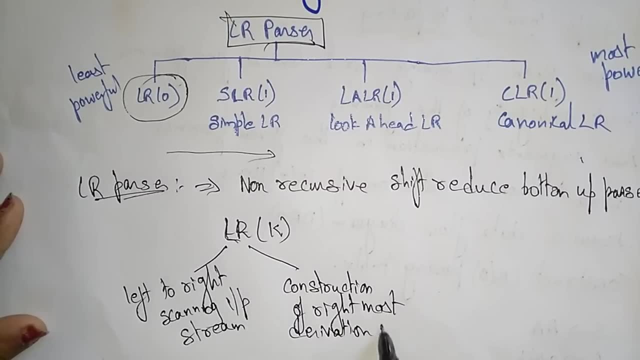 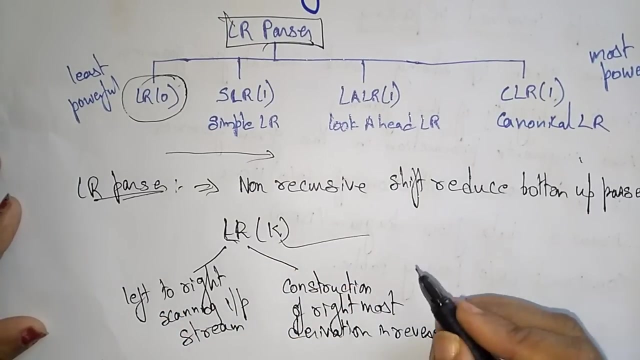 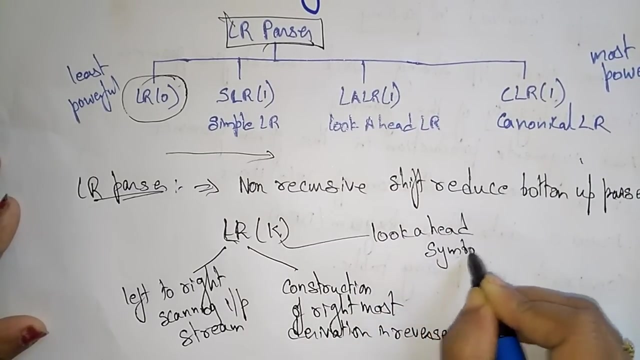 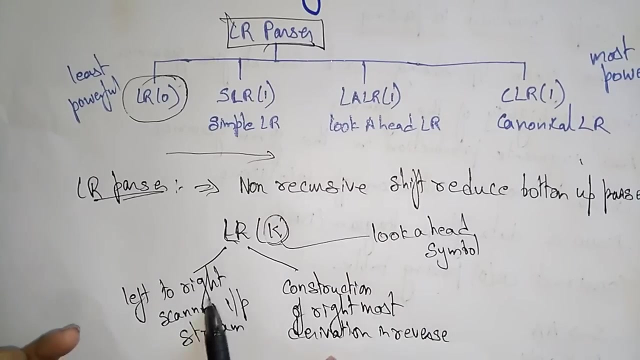 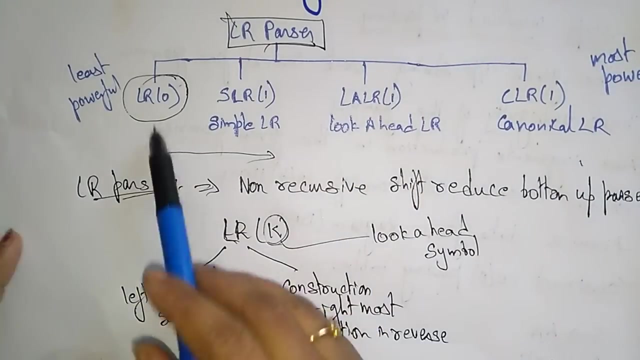 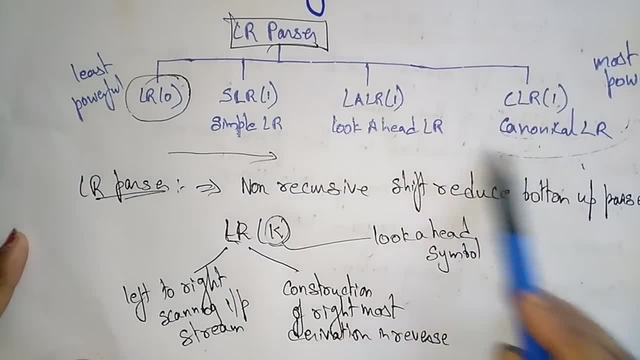 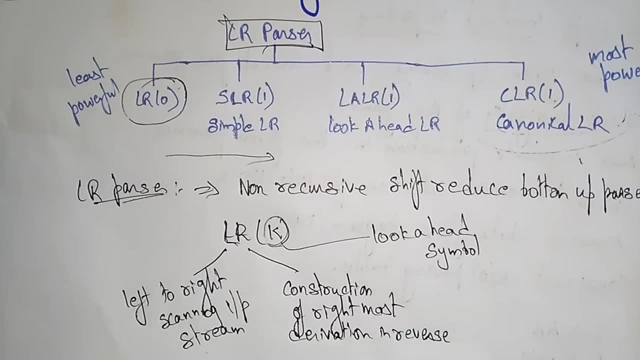 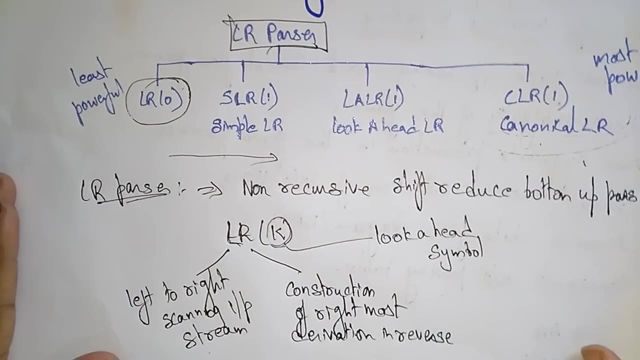 So the canonical LR we already used, we will use in this examples while we are discussing. So the main three available algorithms for constructing LR parser is LR0, CLR1, LALR1.. Okay, now let's see what are these terms are. 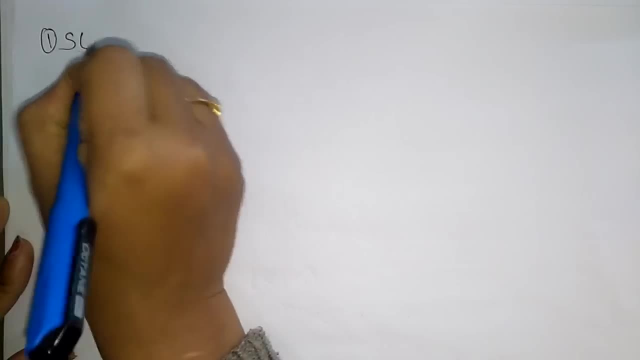 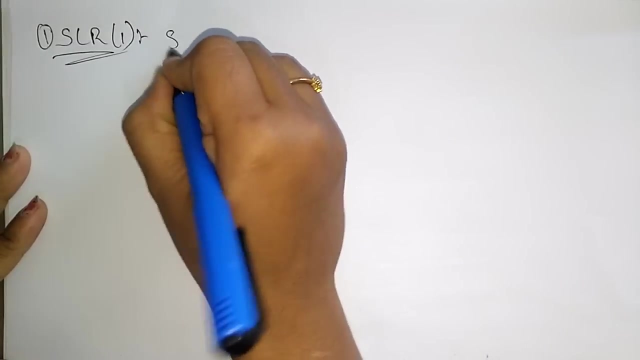 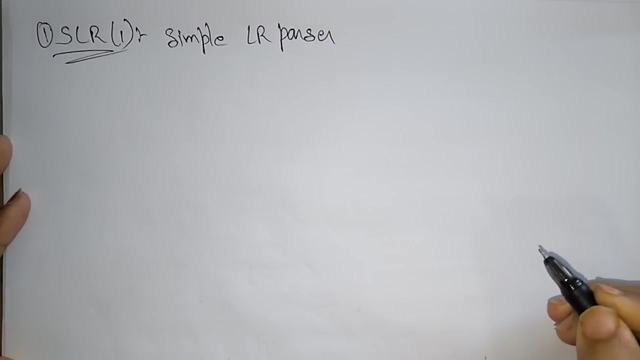 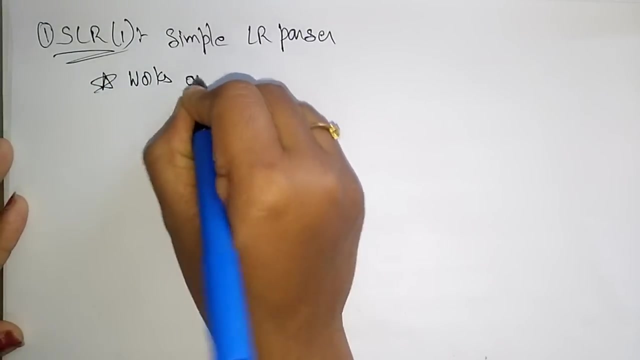 SLR1.. What is SLR1?? So SLR1 is nothing but the simple LR parser. S stands for simple, Simple LR parser And it is works on smallest class of grammar. Let me write the points so that it is useful for you. 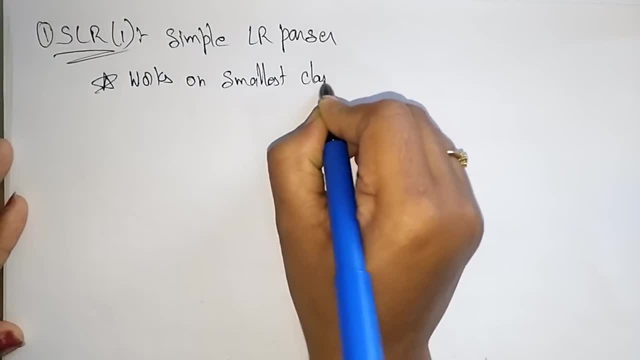 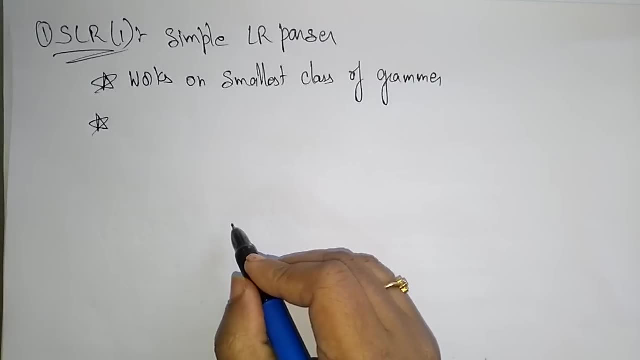 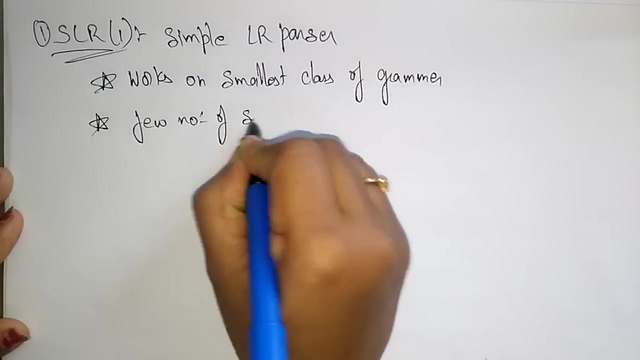 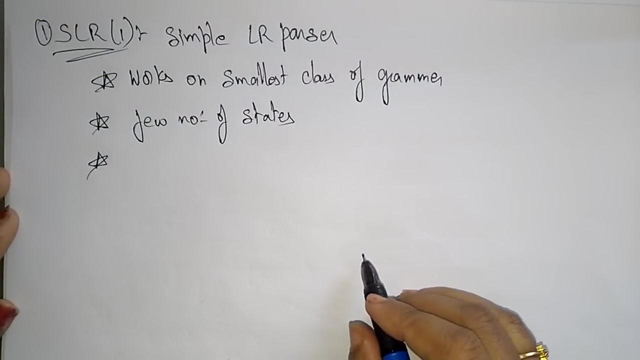 Works on smallest class of grammar And SLR has few number of states, hence very small table. So it's having only few number of states, So it contains very small table when compared to the other LR0. And it is a simple and fast construction. SLR is simple and fast construction. 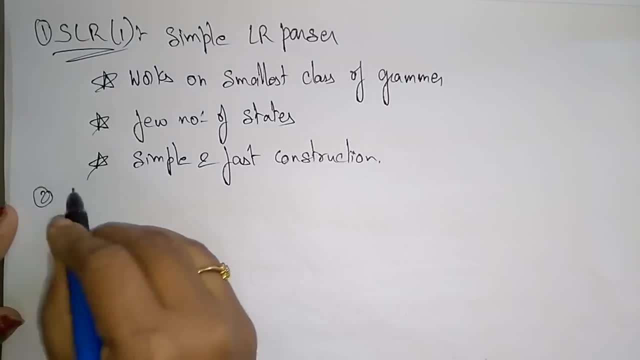 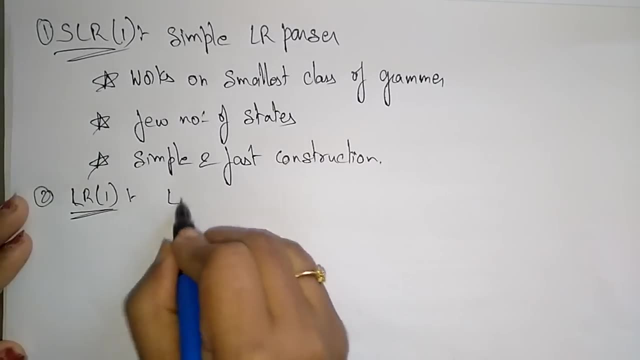 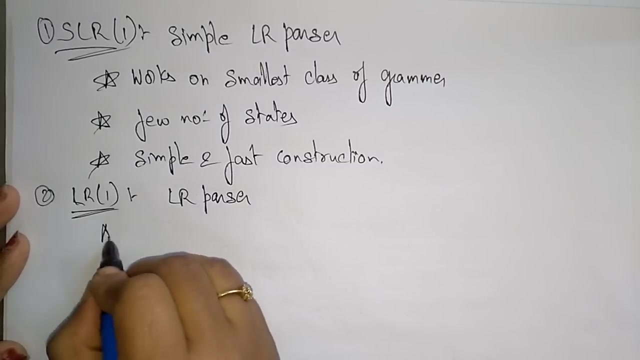 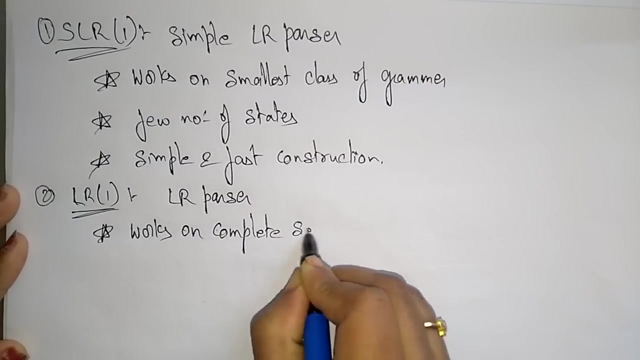 So these are the features of this simple LR parser. Now let's see the next one, LR1.. Let's take LR1.. That is nothing but LR parser. So it works on a complete set of LR1 grammar. Works on complete set of LR1 grammar. 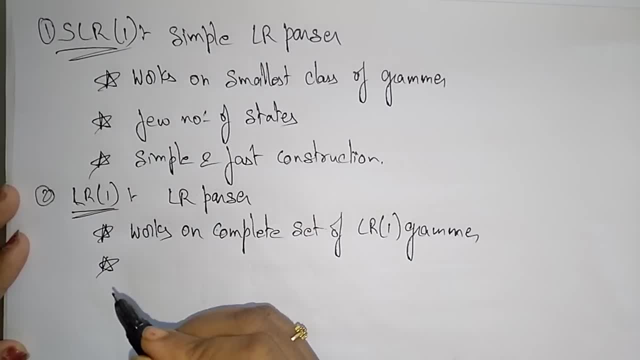 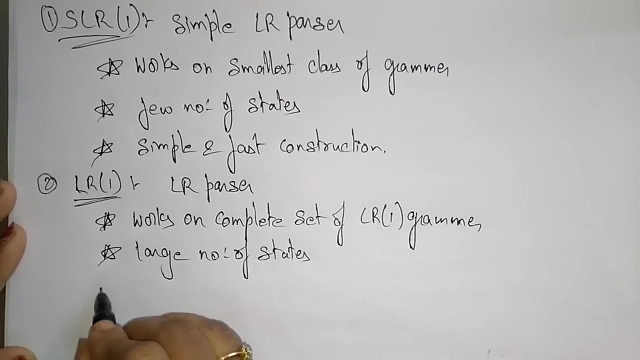 And it generates large table and large number of states will be there. So here there are few number of states and LR1 is having the large number of states. Whenever the states are increasing, obviously the table is also becomes big. And if the table is more, which generates a large table, means slow construction. 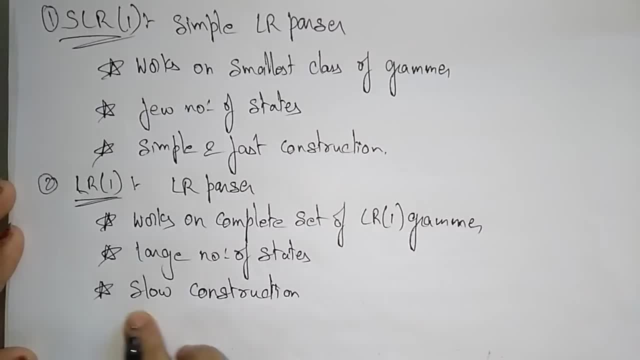 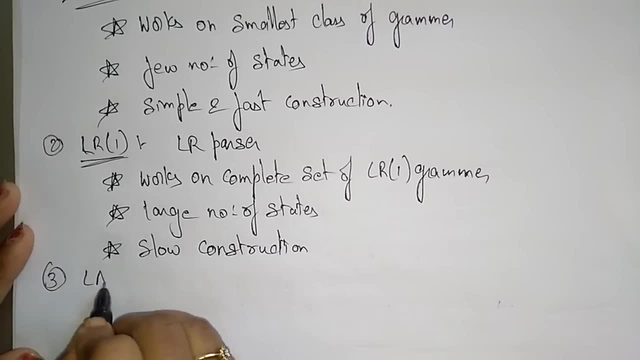 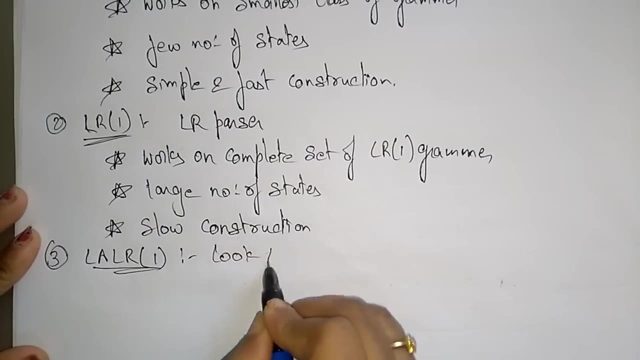 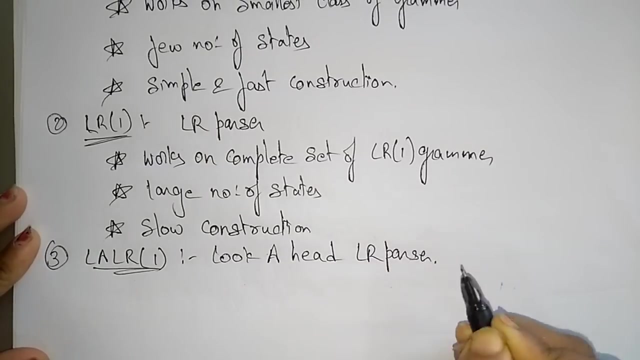 Few tables, few state means only the simple and fast construction, Whereas LR is having the slow construction. Now coming to the next available algorithm, that is LALR. LALR is nothing but look ahead, LR parser. So it works on intermediate size of the grammar. 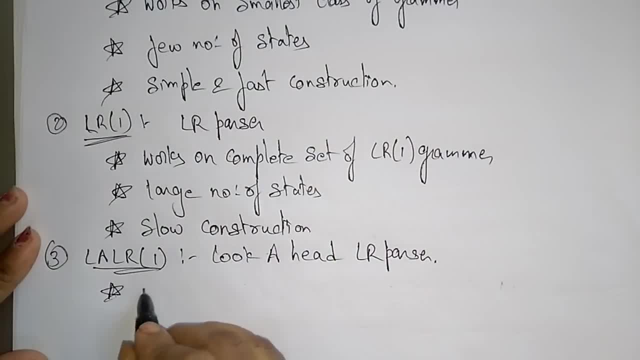 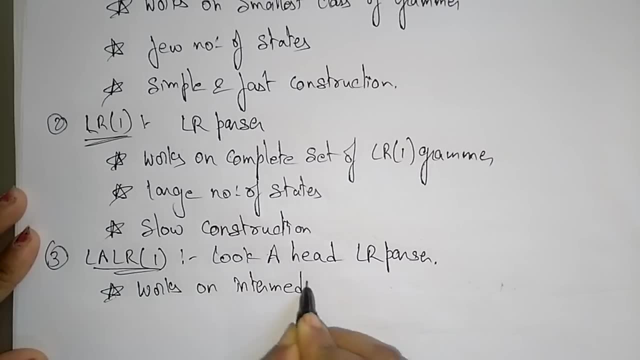 Here, LR works on the complete set of LR grammar, Whereas LALR works on intermediate size of grammar, And number of states are same as SLR. So then it is simple and fast to construct: Number of states are same as SLR1.. 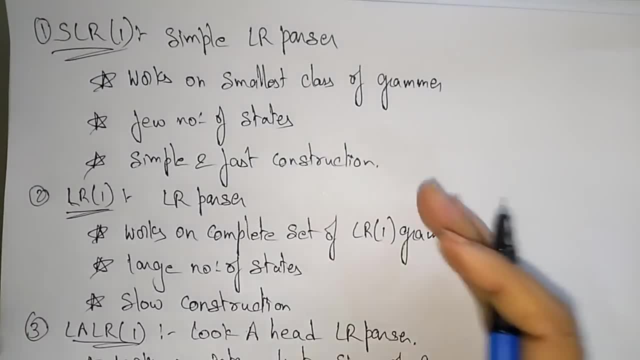 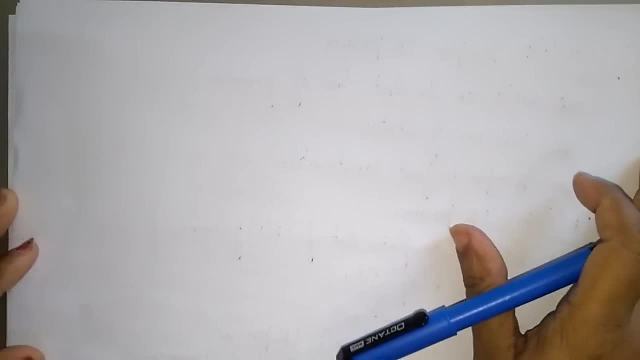 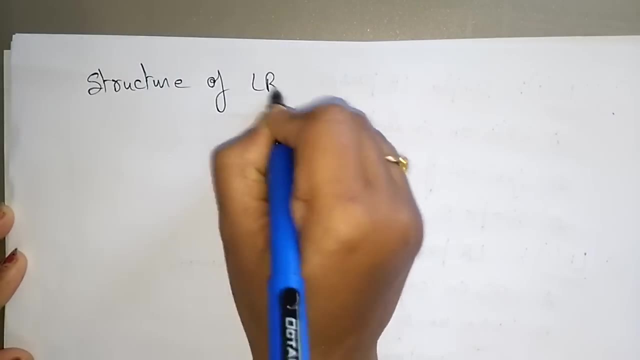 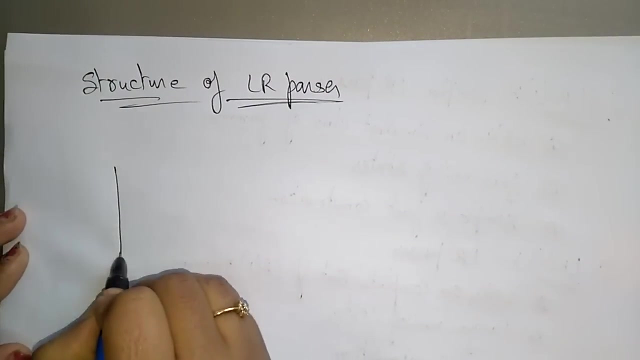 So just remember these points and the features of SLR, LR and LALR. Let's see the structure of LR parser. Later we will see the examples how the LR is going to be construct. Structure of LR parser. So LR parser consisting of stack which holds the data. 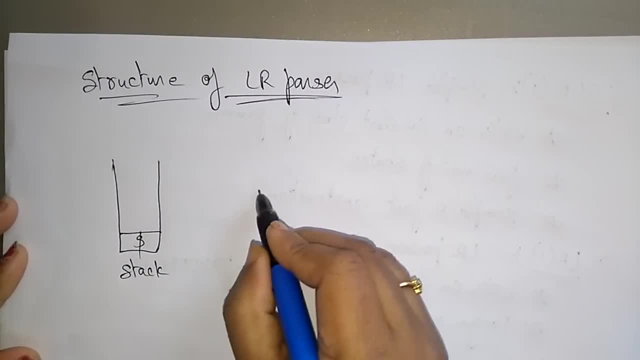 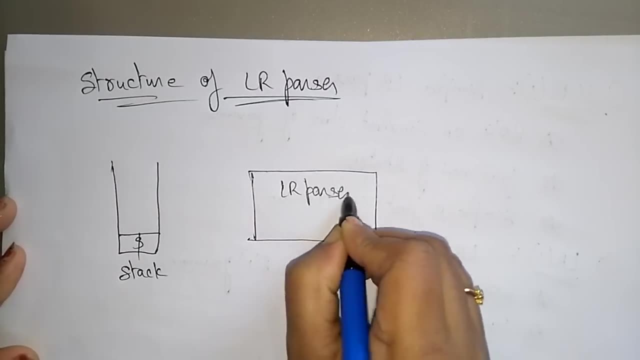 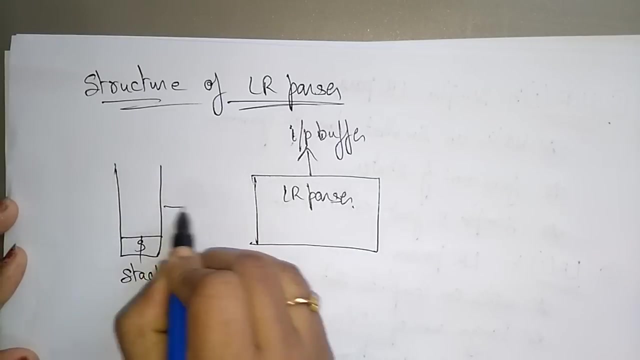 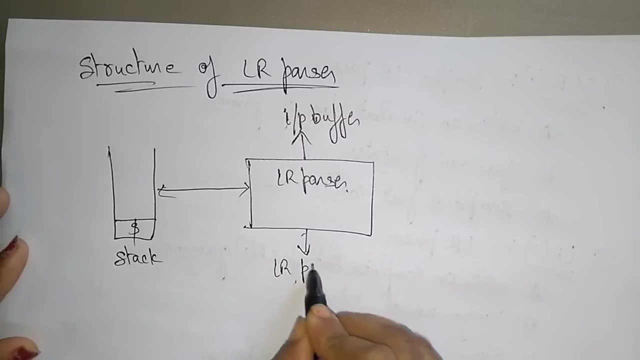 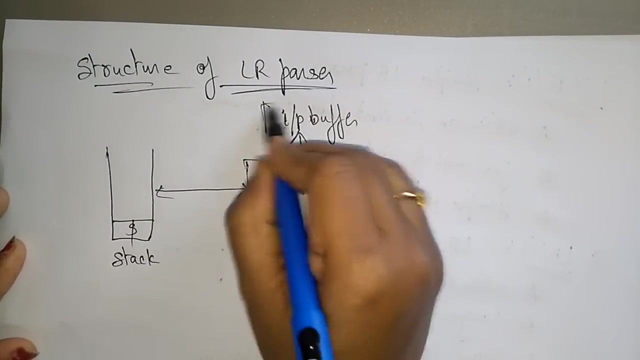 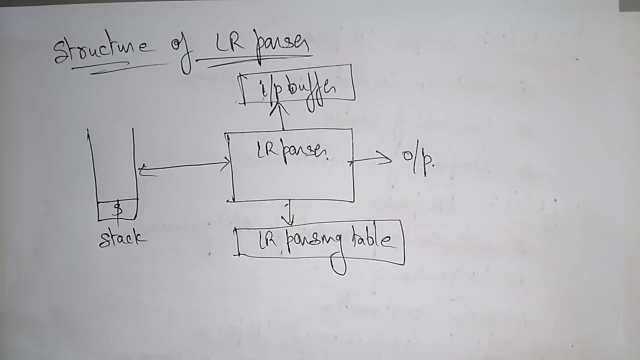 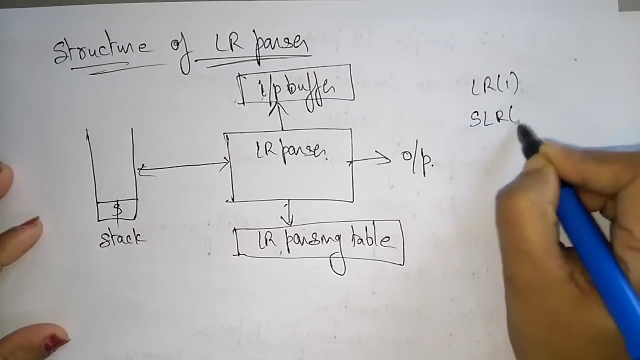 stack starts with the empty symbol and it consisting of LR parser and input buffer- LR parsing- table output. this is structure of LR parser actually. so, whatever the parsers you are taking, that is LR 1 and SLR 1, LR 0 or SLR 1, whatever it may be, and SLR 1 see LA LR 1. so for all these, 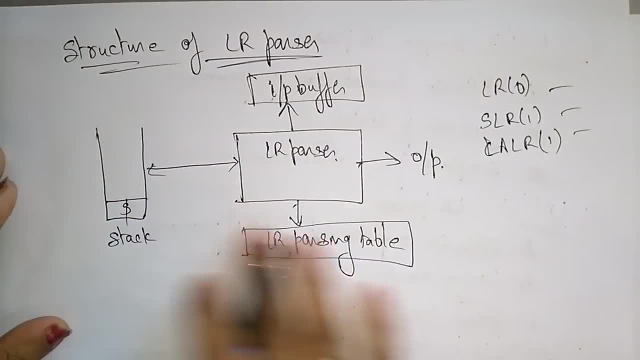 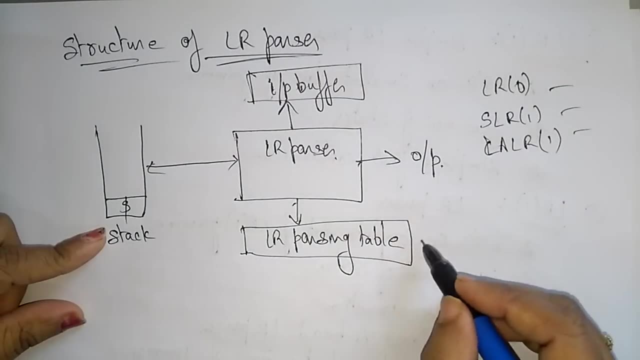 available algorithms, this structure is the same. so for all these available algorithms, this structure is the same. so for all these available, so they are- use the same stack, the same input buffer and LR parser. everything will be the same, but only difference is a parsing table each algorithm is having. 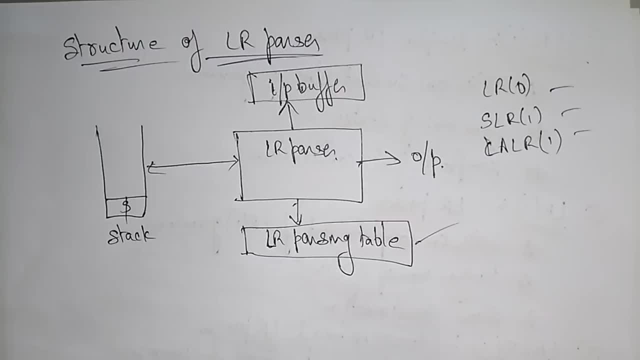 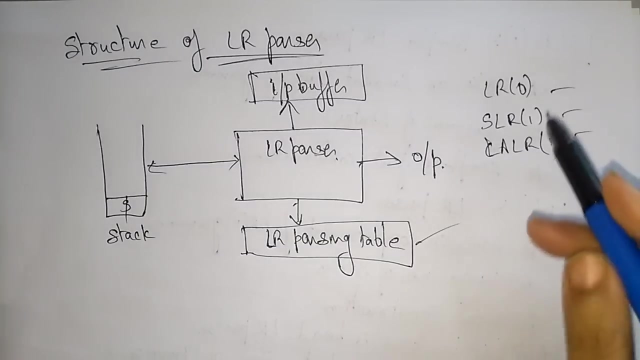 their own type of parsing table. okay, so, whenever you are solving the problems of LR parsers, okay, the stack implementation, input buffer and construction of LR parser, everything is same for all the algorithms. but the only difference in this here is a LR parsing table. so the only difference is the same for all the 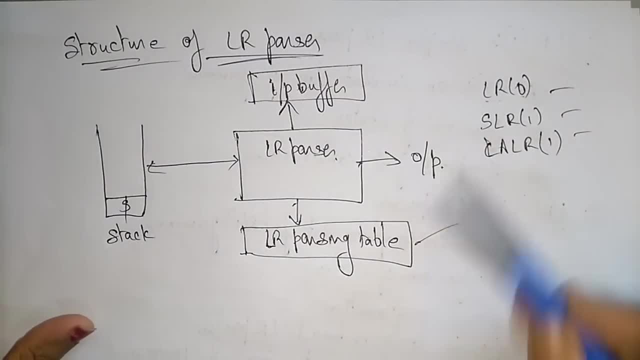 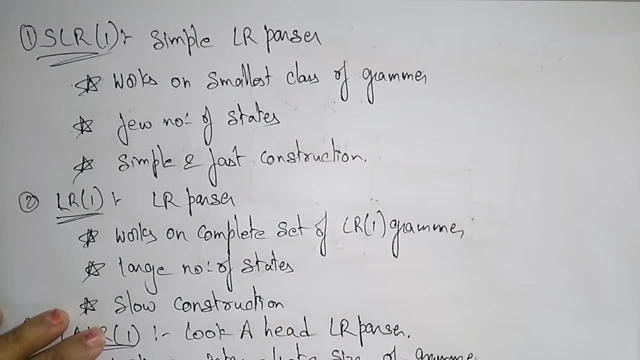 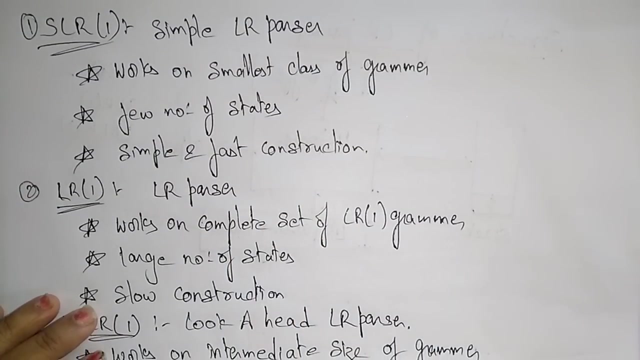 LR parser, each having their own technique. because in the parsing table itself, whatever the features, you are seeing that here in the- to construct the parsing table you need the states. so as LR is having only few states and the construction of the table is also constant, only few state- okay means the. 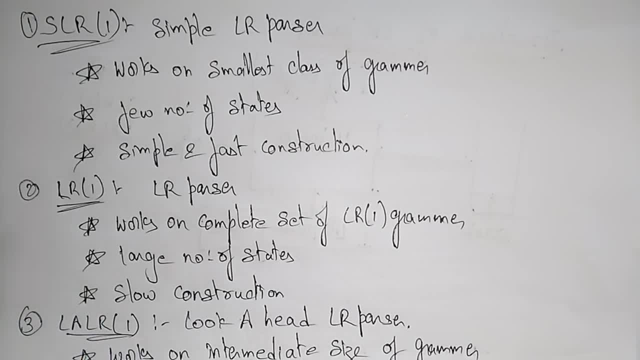 construction is very lesser: a few number of states. hence very small table is required, SLR equal to any small table and SLR requires very small table. and whereas LR requires large number of states, means large table is right now. so this is loved. based out of ОнTL is definitely tone to shape data in the file lot, see 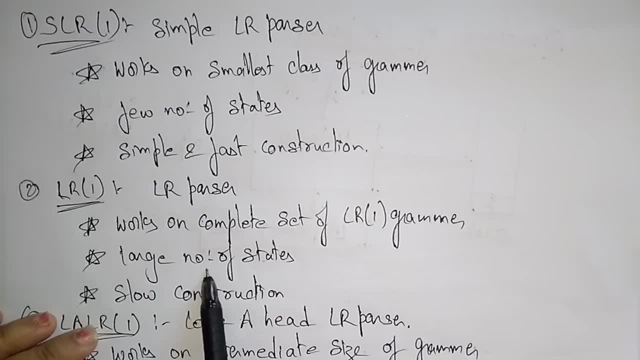 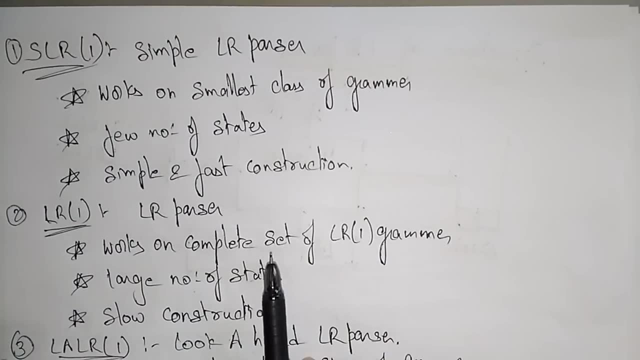 promise on what are you getting from sólo such cái mass always to be when we get LR parser facebookcom first. never see any of those stars previously. did now tour where we specialtyえ table is required and lalr is having the same states whatever the slr is having, okay, so 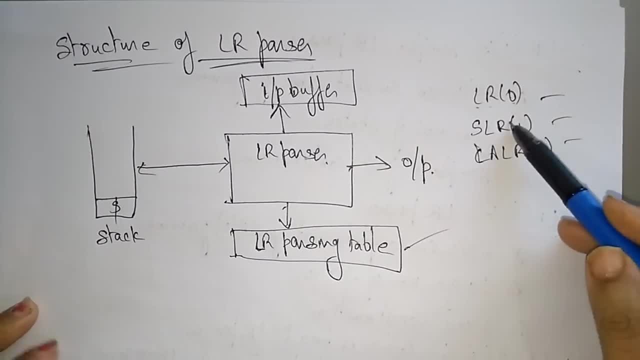 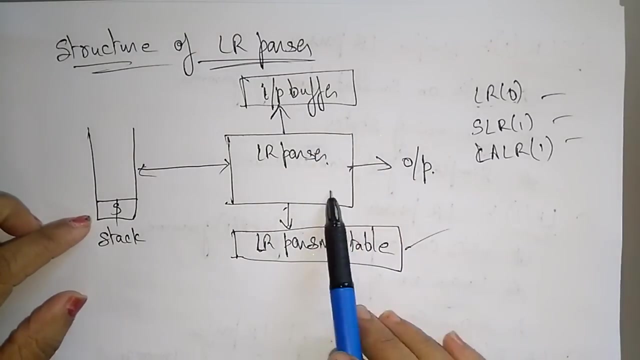 everything, uh, whatever the grammar that is present, uh, that is used in slr, slr, uh, la, lr, everything is the same. the only difference here is the parsing tables, whatever they are using. so lr parsing algorithm requires a stack input buffer and lr parsing table from all these parse. 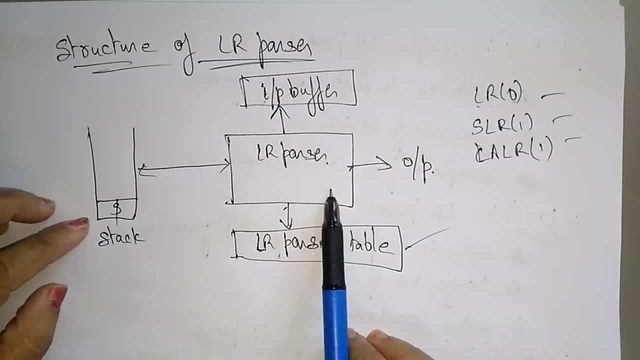 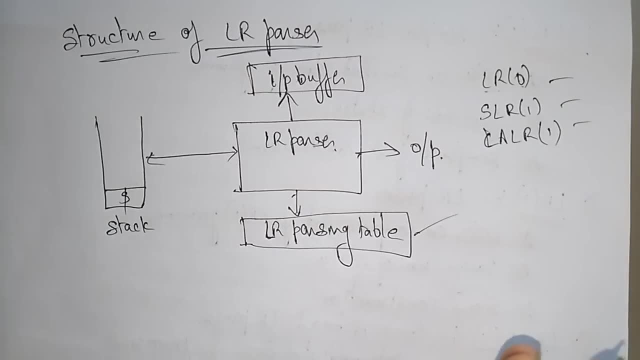 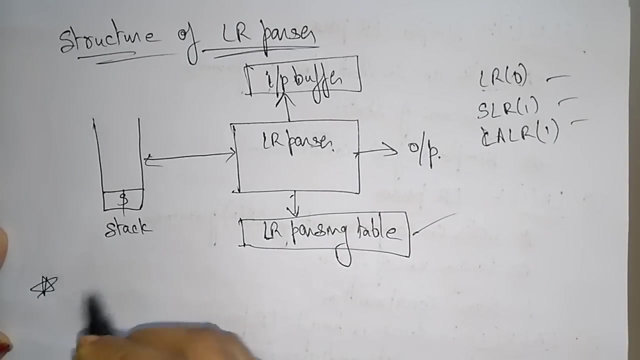 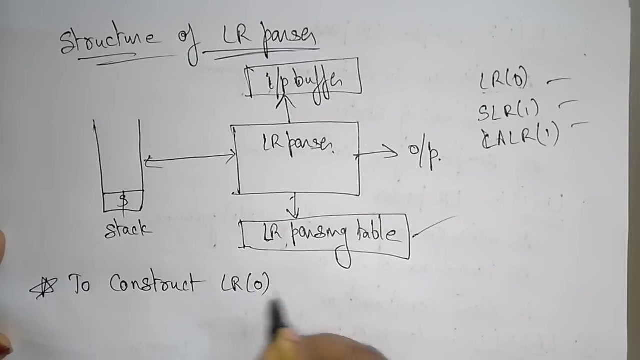 table. so the stack and input buffer lr parser algorithm is same but only difference is parsing table. so to construct lr of 0 and slr 1 tables we use canonical collection of lr 0 item. so these points. you just remember that to construct lr of 0 and slr of 1, if you want to construct lr of, 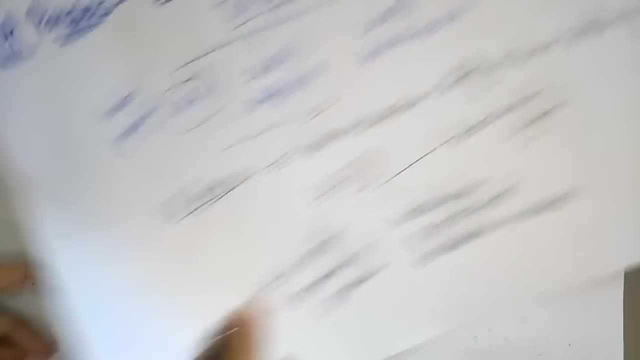 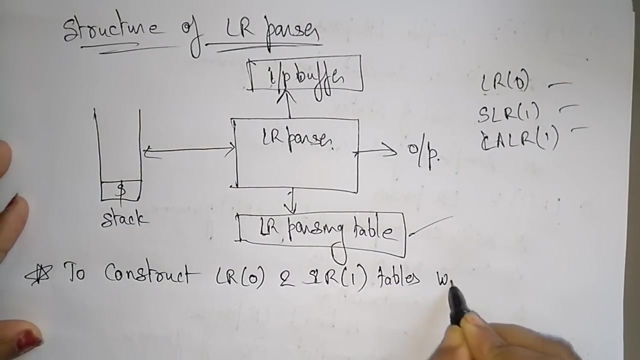 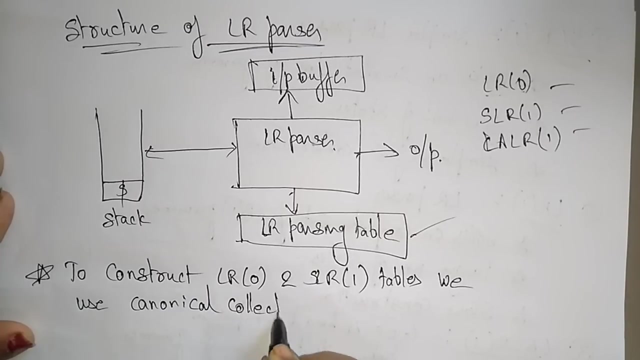 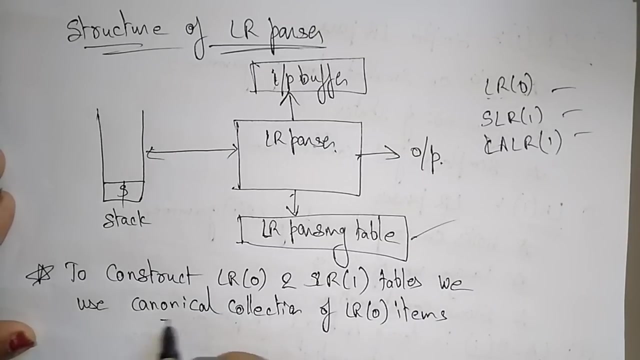 0 and slr 1, the first two items. okay, whatever, here it is present- the first two items: lr of 0 and slr 1 tables. we use canonical collection of lr 0 items, so to construct a table it requires the canonical collection of lr 0 items. so just, uh, remember this word, so it will be helpful. 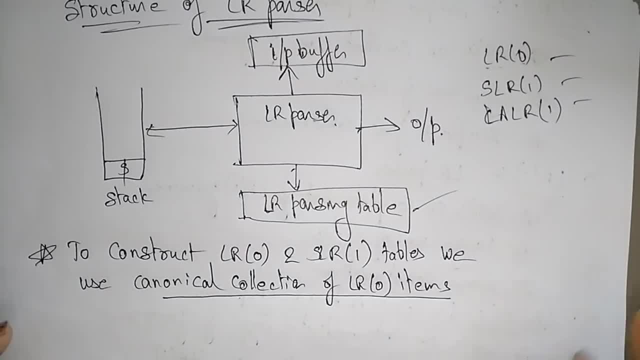 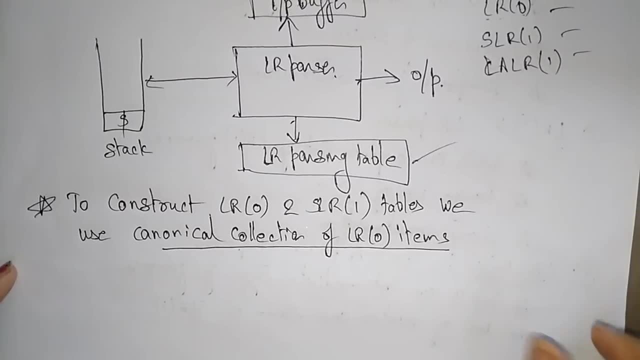 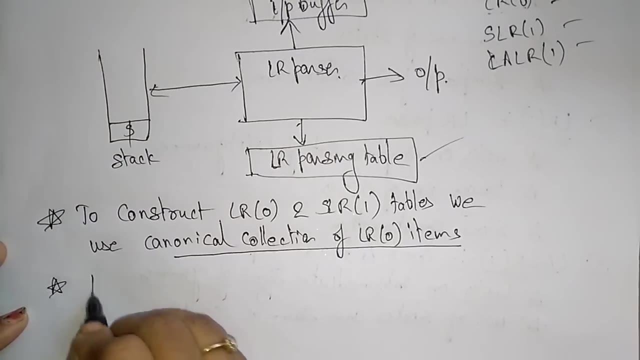 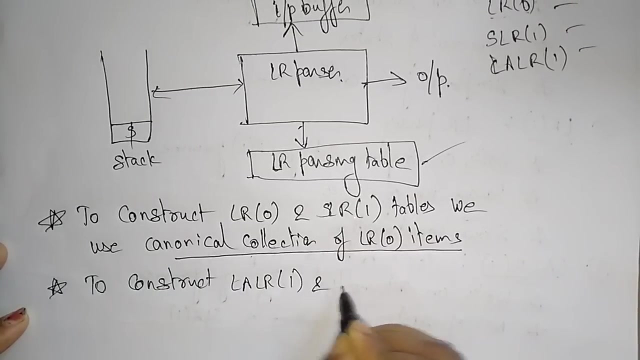 to you while you're uh constructing the tables. so, to construct lr of 0 and slr 1 tables, we use canonical collection of lr 0 items. so what are this canonical collection of lr 0 items? you will see in the examples. okay, and next, uh, to construct l, a, lr of 1 and c lr of 1 tables, the remaining two. 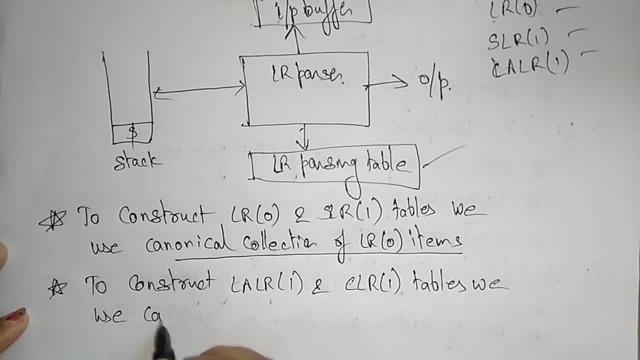 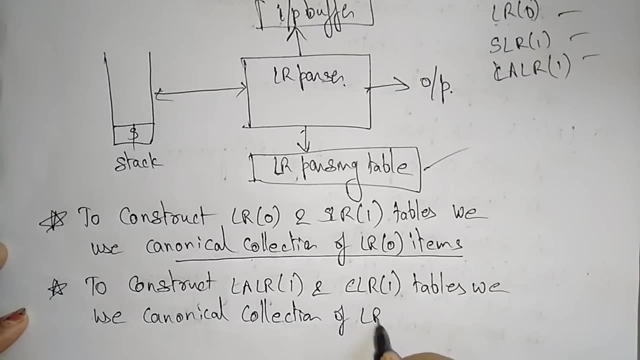 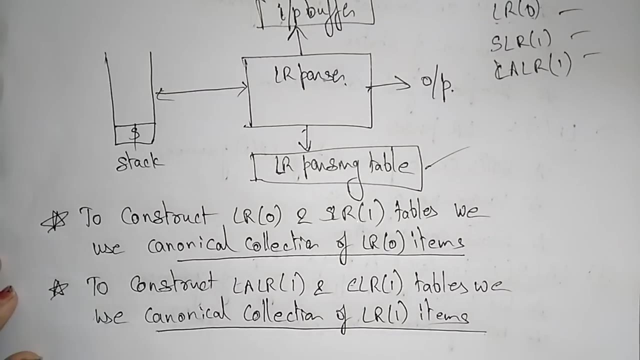 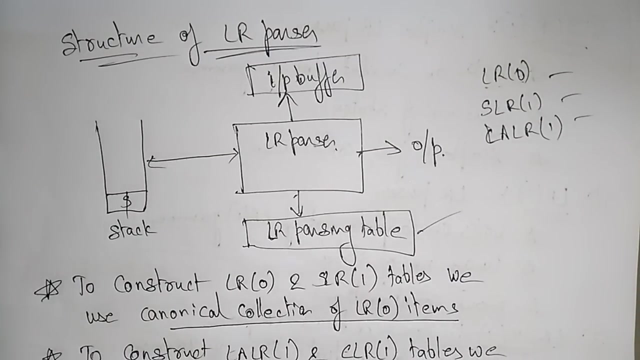 we use canonical collection of canonical collection of lr 1 items. so for constructing l a, lr and c lr, we use the canonical collection of lr 1 items. okay, so this is just an introduction part of the lr parser. how the lr parser having the different uh algorithms- lr 0, slr, c, l, a, lr and.